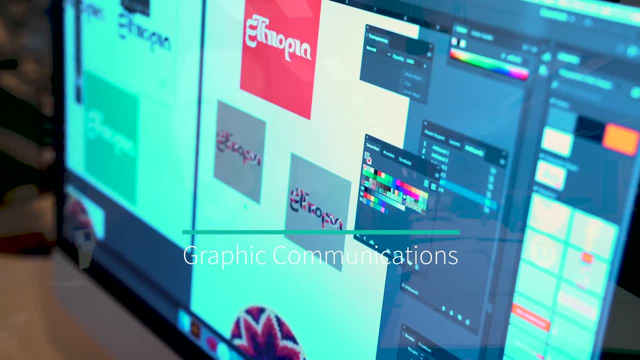 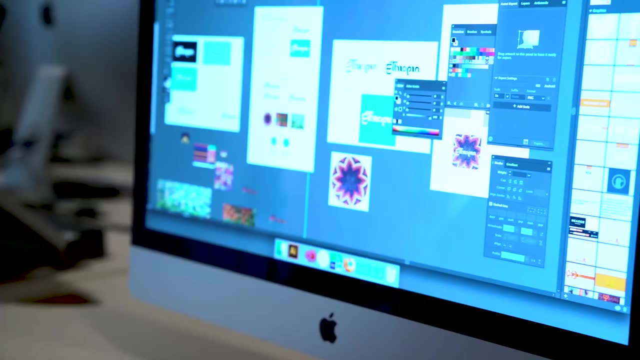 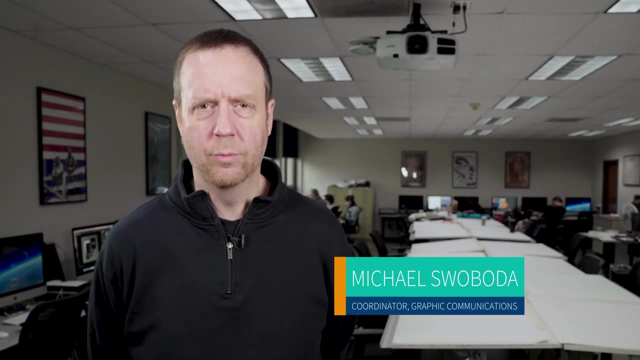 We have three degree options. We have an Associates of Fine Arts and we have two options within the Associate of Applied Science, and each one of the degrees are around 65 credit hours. Students can start in the fall of a year and in two years finish and with that they they leave with a wonderful portfolio- a lot. 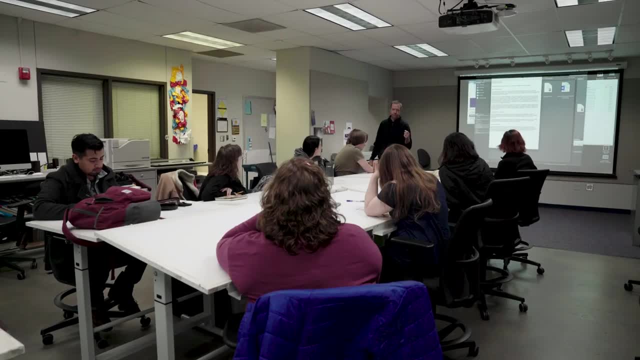 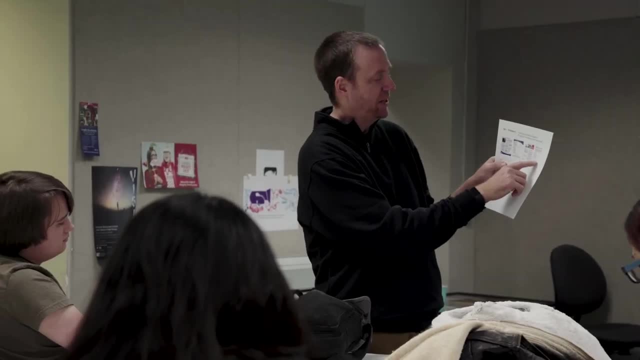 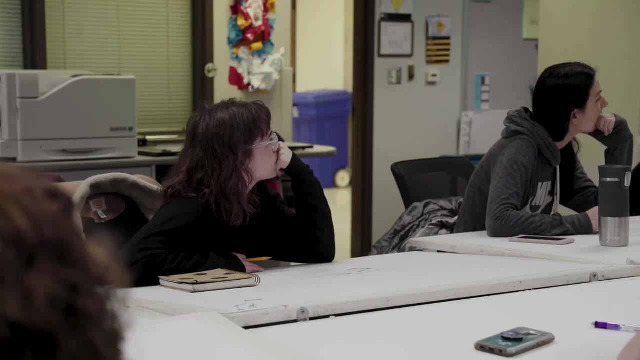 of interviews and interview skills and, in many cases, an internship experience ready for the workplace or for transfer to an accredited four-year institution. Just the setting and the tab organization and the hierarchical structure of a list with different kinds of qualities and being able to handle that in a professional way is like a golden ticket to success. I think we've 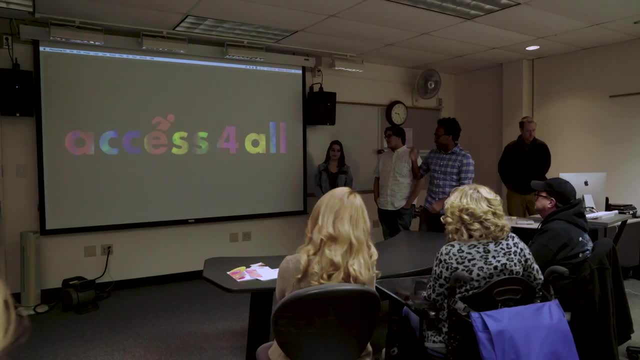 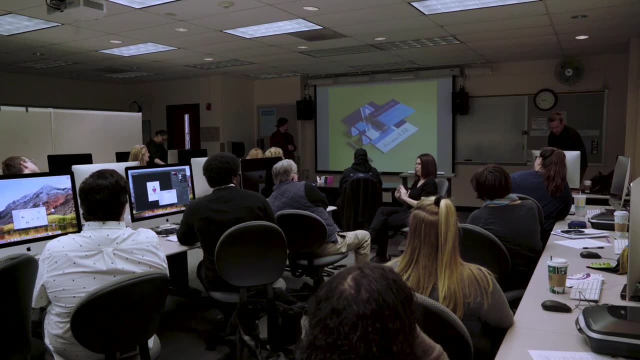 done a wonderful job of designing a program that positions students to be ready for what's going on in graphic design and graphic communications today. We combine web design and motion design and a lot of cutting-edge technologies with the tradition of graphic design, For instance. we really believe in the 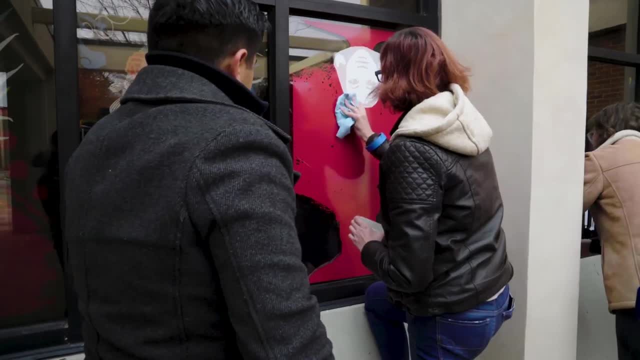 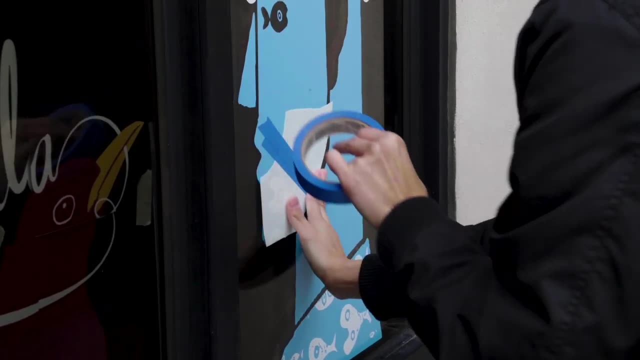 foundation of graphic design. We believe in the foundation of graphic design, We believe in the foundation of drawing and the foundation of outstanding typography and the foundation of illustration. We combine all those things with, I think, good classroom citizenship skills and interview skills, the ability to 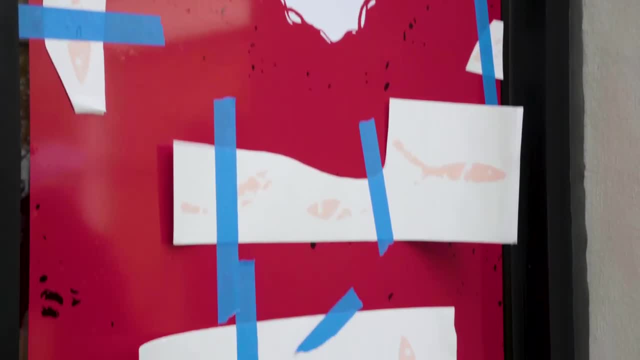 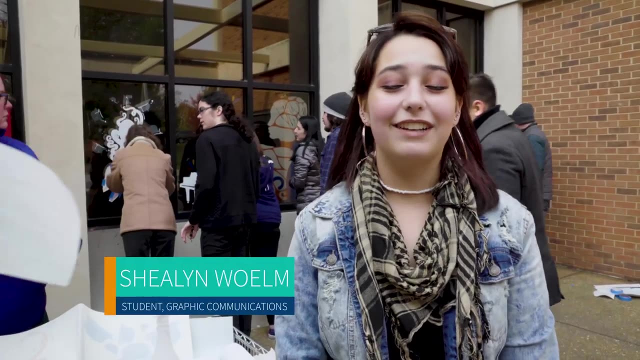 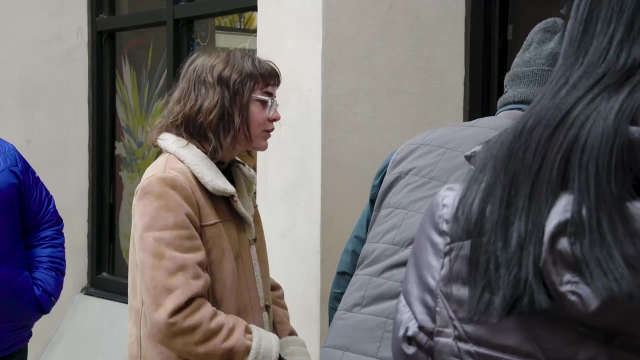 interview for prospective employment. The favorite thing about the program would probably be all the different students that you just get to interact with and also the professors. They're very helpful and some of them are really great and down to earth and they just really guide you into helping you figure out what you want to do and where you want to go in life. 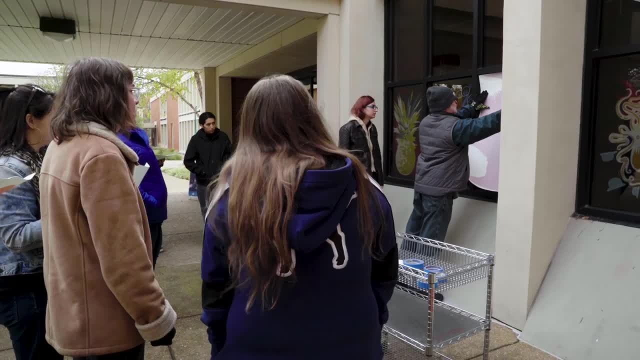 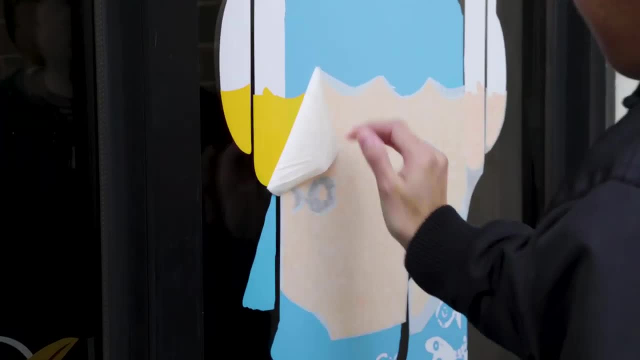 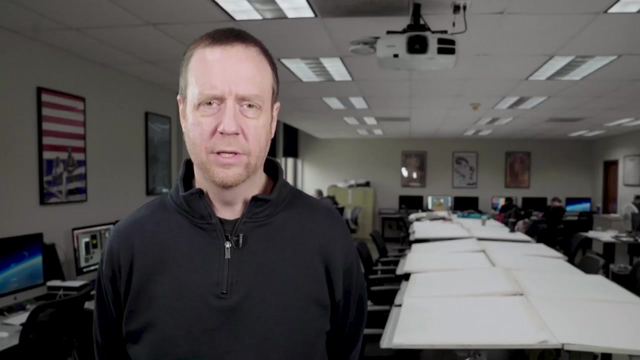 We have a blue tape to position them where they go, okay. We have a blue tape to position them where they go, okay. Well, our students sometimes come to our program with very little skills and Photoshop, Illustrator, InDesign, After Effects. They may draw a little bit, but they have no background in typography or into the standards of graphic design. So we take students in a very raw state and, in a very short period of time, transforming them into successful graphic designers. 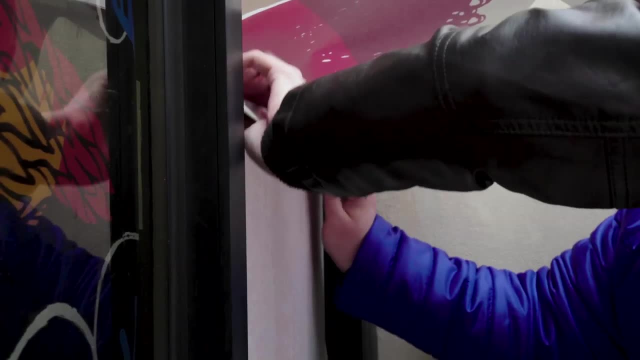 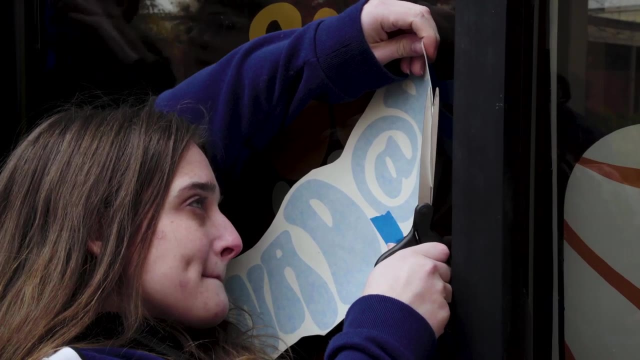 In recent years we've just seen so many of our students go on to so many very fine colleges and universities and win so many interesting jobs that they don't even know they're doing and be a part of outstanding internship opportunities. The students that come in are, by and large,